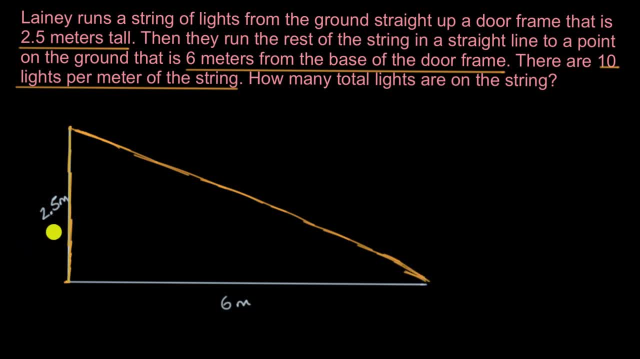 So the yellow right over here, that is the light, And so we need to figure out how many total lights are on the string. So the way I would tackle it is: first of all I want to figure out how long is the total string. 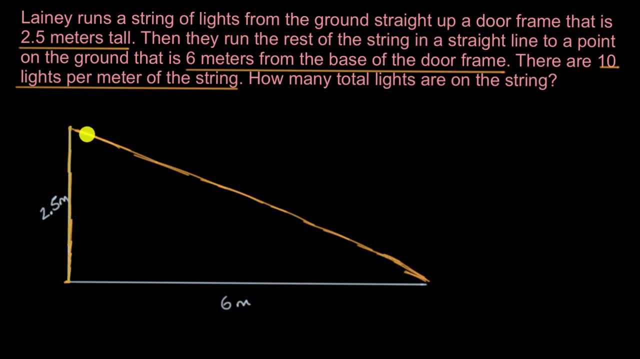 And to figure that out, I just need to figure out: okay, it's going to be 2.5 plus. whatever the hypotenuse is of this right triangle, I think it's safe to assume that this is a standard house where doorframes are at a right angle to the floor. 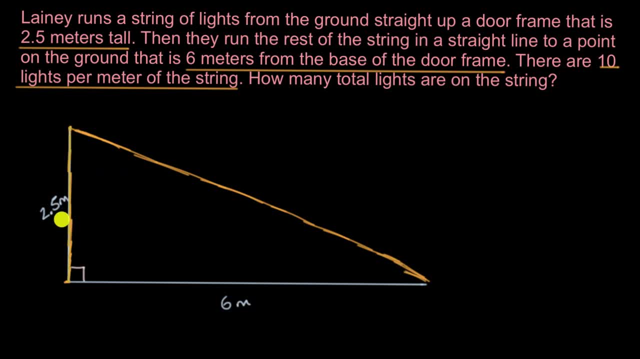 And so we have to figure out the length of this hypotenuse, And if we know that, plus this 2.5 meters, then we know how long the entire string of lights are, And then we just have to really multiply it by 10. 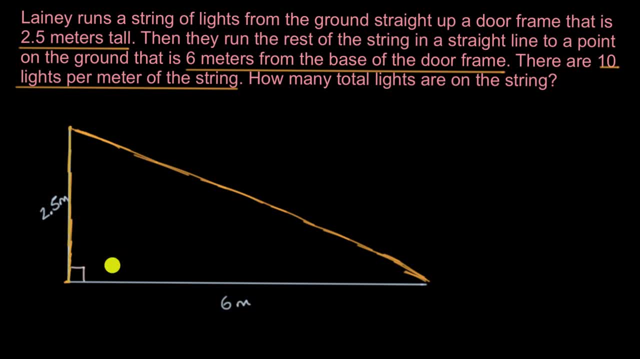 because there's 10 lights per meter of the string, And then we just have to really multiply it by 10, because there's 10 lights per meter of the string. So let's do that. So how do we figure out the hypotenuse here? 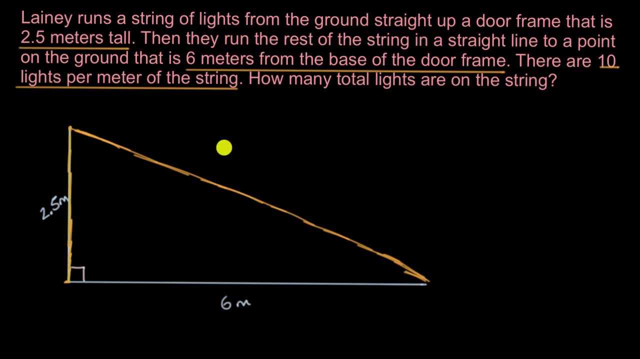 Well, of course, we would use Pythagorean theorem. So let's call this, let's call this h for hypotenuse. We know that the hypotenuse squared is equal to 2.5 squared plus six squared, So this is going to be equal to 6.25. 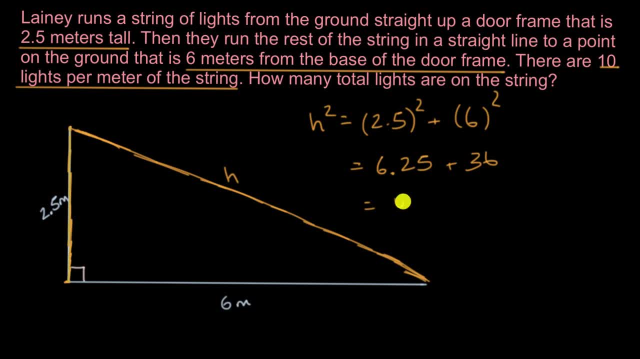 plus 36,, which is equal to 42.5.. which is equal to 42.5.. Or we could say that the hypotenuse is going to be equal to the square root of 42.25.. And I could get my calculator out at this point. 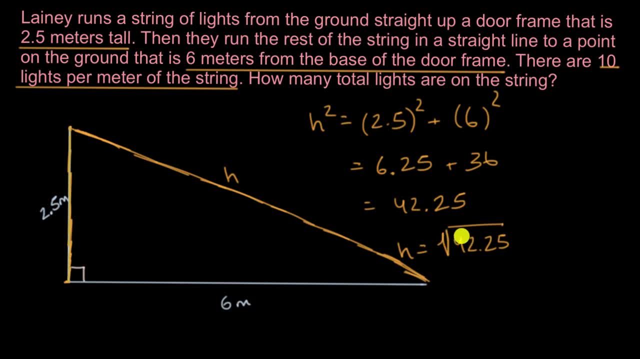 but I'll actually just keep using this expression to figure out the total number of lights. So what's the total length of the string? We have to be careful here. A lot of folks would say: oh, I figured out the hypotenuse. 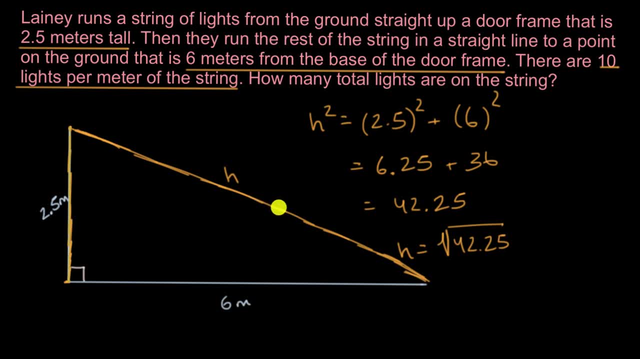 Let me just multiply that by 10.. In fact, my brain almost did that just now, But we got to realize that the entire string. But we got to realize that the entire string is the hypotenuse plus this 2.5.. 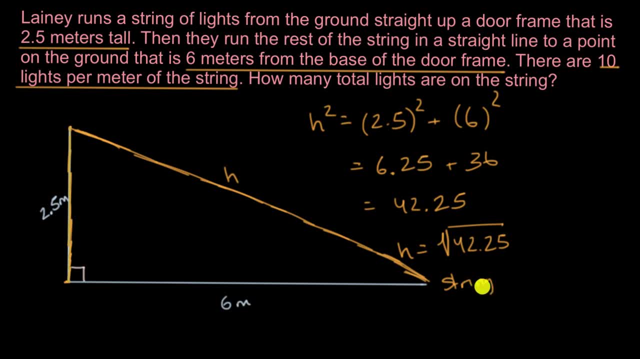 So the whole string length. let me write it this way: string length is equal to 2.5. string length is equal to 2.5 plus the square root of 42.25.. plus the square root of 42.25.. 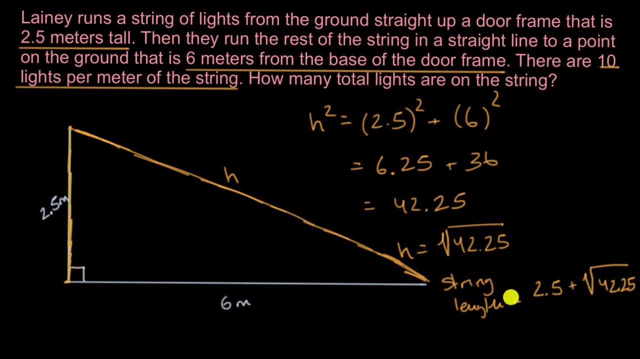 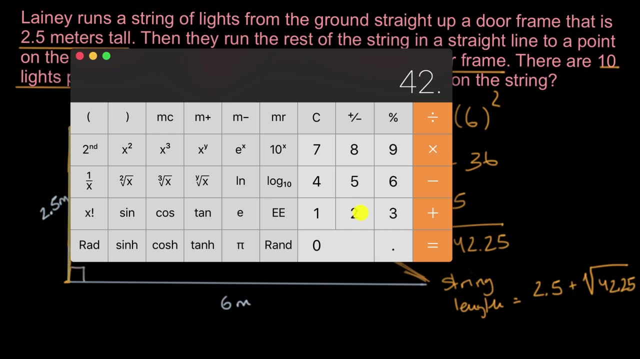 And then we would just multiply that times 10 to get the total number of lights. So now let's actually get the calculator out. So we have 42.25, and then we were to take the square root of that gets us to 6.5,. 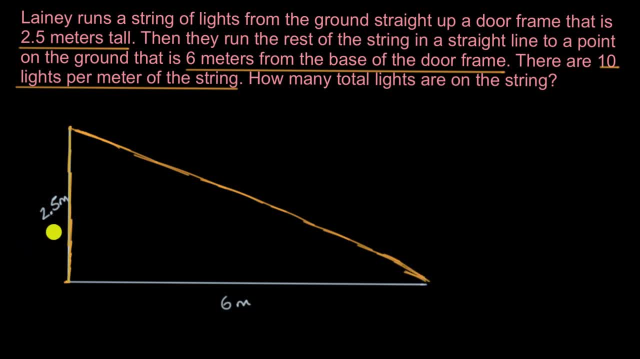 So the yellow right over here, that is the light, And so we need to figure out how many total lights are on the string. So the way I would tackle it is: first of all I want to figure out how long is the total string. 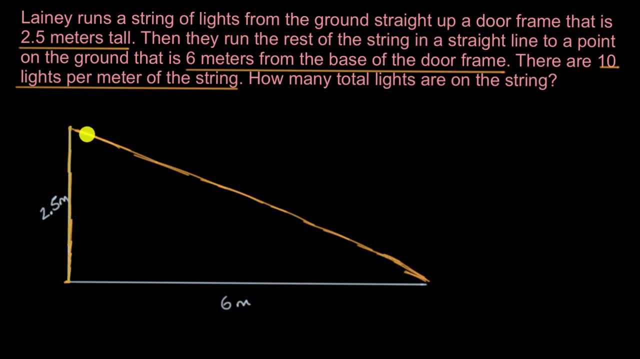 And to figure that out, I just need to figure out: okay, it's going to be 2.5 plus. whatever the hypotenuse is of this right triangle, I think it's safe to assume that this is a standard house where doorframes are at a right angle to the floor. 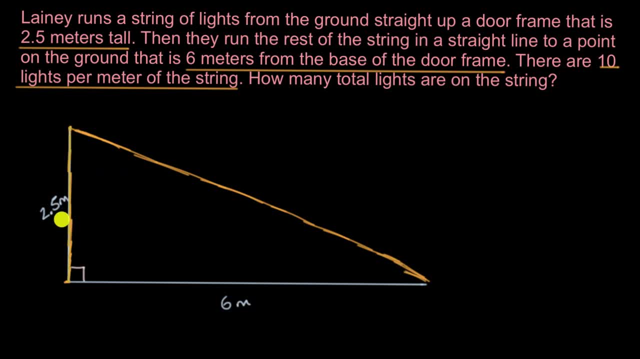 And so we have to figure out the length of this hypotenuse, And if we know that, plus this 2.5 meters, then we know how long the entire string of lights are, And then we just have to really multiply it by 10. 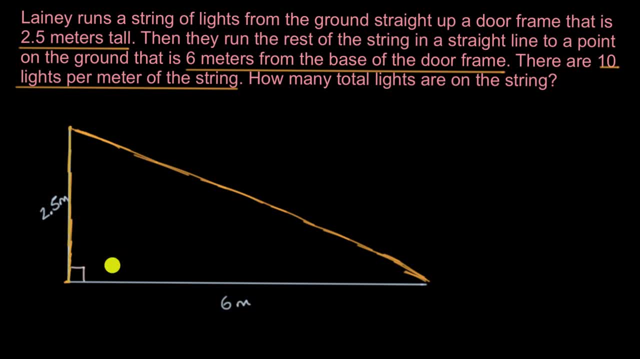 because there's 10 lights per meter of the string, And then we just have to really multiply it by 10, because there's 10 lights per meter of the string. So let's do that. So how do we figure out the hypotenuse here? 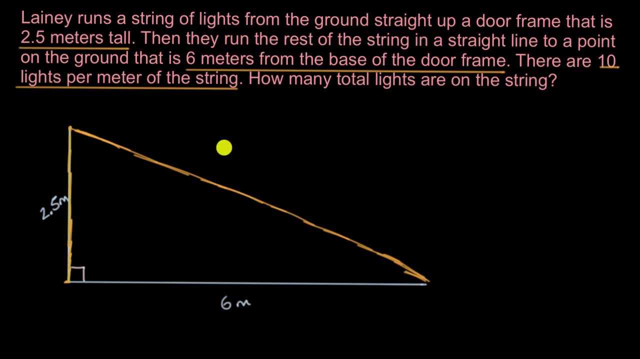 Well, of course, we would use Pythagorean theorem. So let's call this, let's call this h for hypotenuse. We know that the hypotenuse squared is equal to 2.5 squared plus six squared, So this is going to be equal to 6.25. 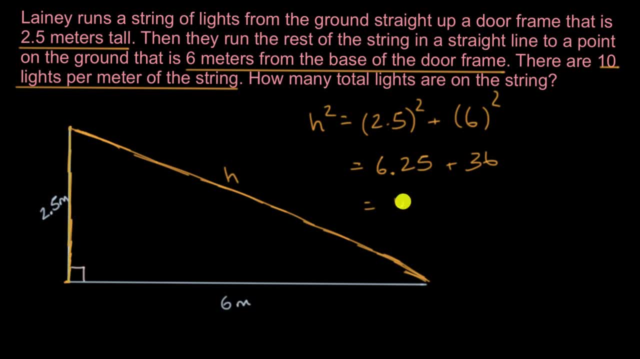 plus 36,, which is equal to 42.5.. which is equal to 46,, which is equal to 42.5.. Or we could say that the hypotenuse is going to be equal to the square root of 42.25.. 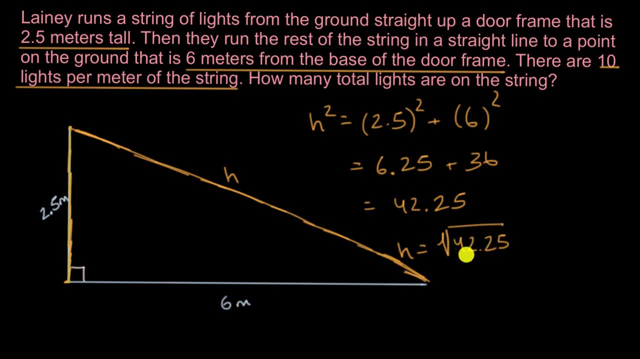 And I could get my calculator out at this point, but I'll actually just keep using this expression to figure out the total number of lights. So what's the total length of the string? We have to be careful here. A lot of folks would say: oh, I figured out the hypotenuse. 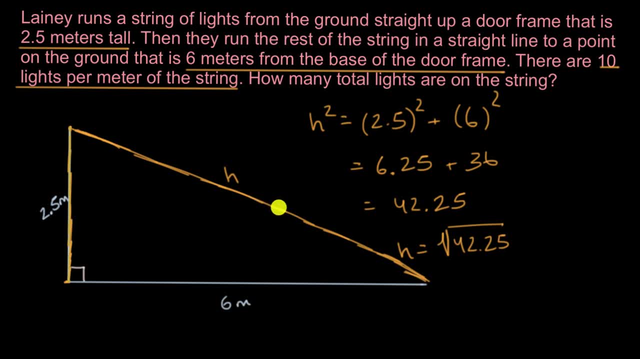 Let me just multiply that by 10.. In fact, my brain almost did that just now, But we got to realize that the entire string. But we got to realize that the entire string is the hypotenuse plus this 2.5.. 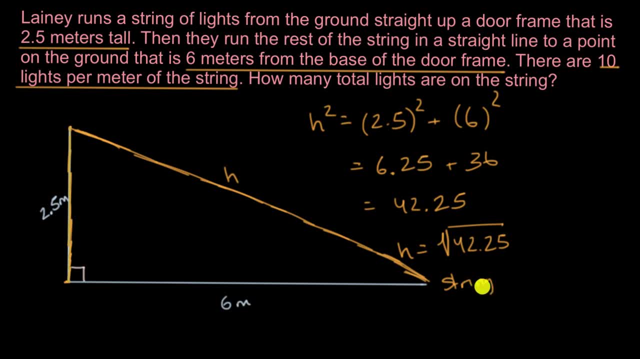 So the whole string length. let me write it this way: string length is equal to 2.5. string length is equal to 2.5 plus the square root of 42.25.. plus the square root of 42.25.. 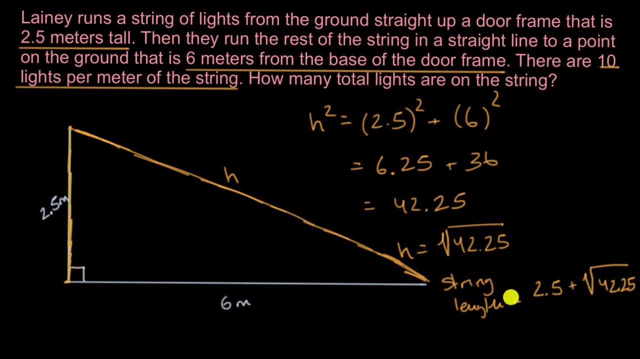 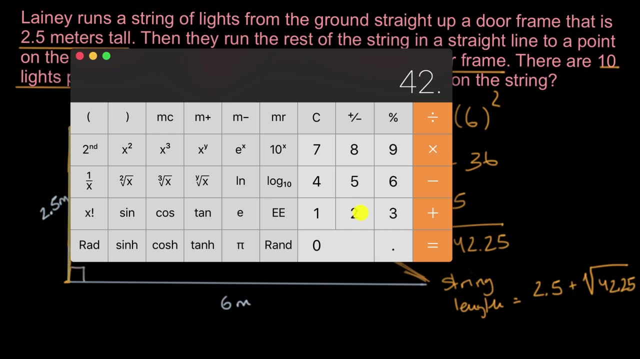 And then we would just multiply that times 10 to get the total number of lights. So now let's actually get the calculator out. So we have 42.25, and then we were to take the square root of that gets us to 6.5,.